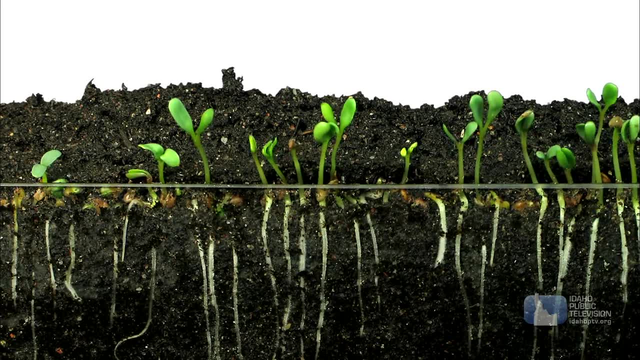 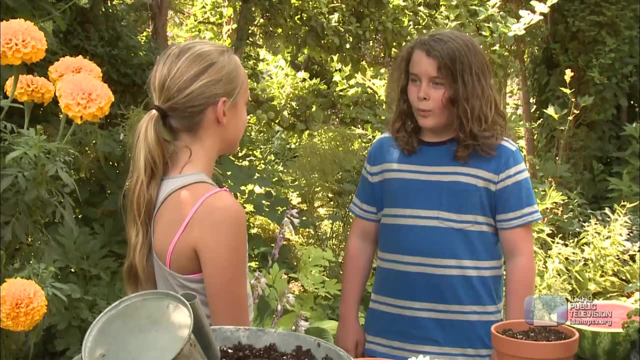 hold them toward the light. Water and minerals travel to the rest of the plant through the stem And finally, the leaves. The leaves are where plants generate their food. Wait, what? What kind of food would plants eat? What kind of food would plants eat? What kind of food would plants eat? 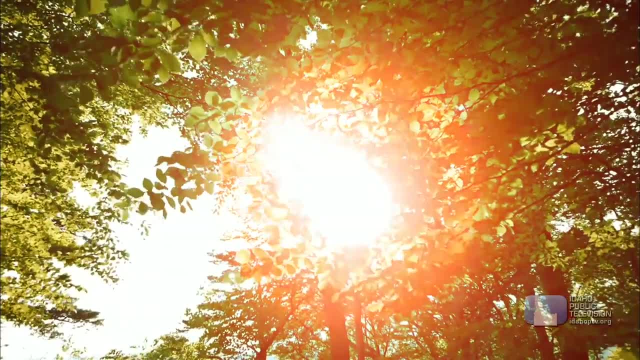 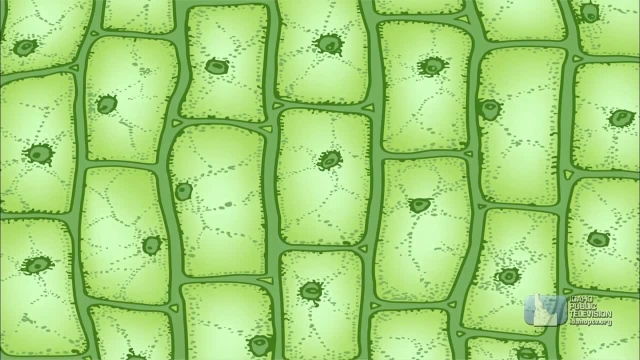 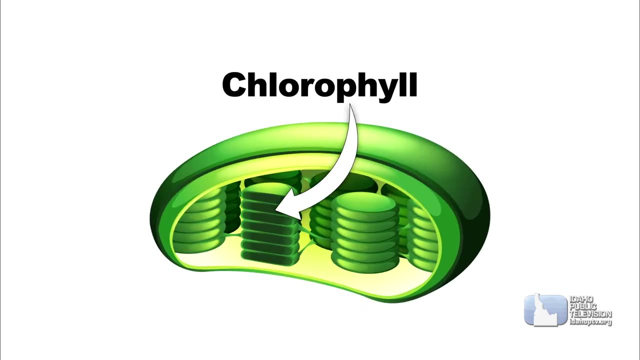 Plants make food by a process called photosynthesis. Plants are made up of tiny plant cells. These cells have tough, thick walls made of a thing called cellulose. Most plants have a substance inside these cells called chlorophyll, And chlorophyll helps plants turn the warmth of the sun into. 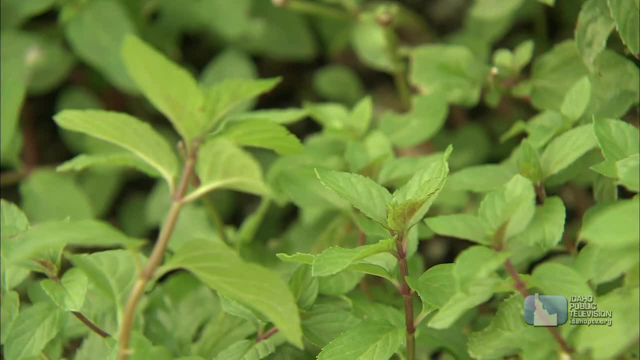 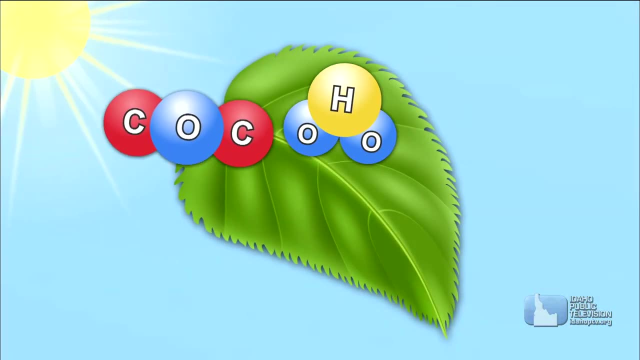 energy. It's also what gives plants their green color. A plant then takes water and minerals from the soil, combines it with gas, carbon dioxide, and then gives it to the plants. A plant then takes from the air and the energy from the sun and makes its own food, And in this process, 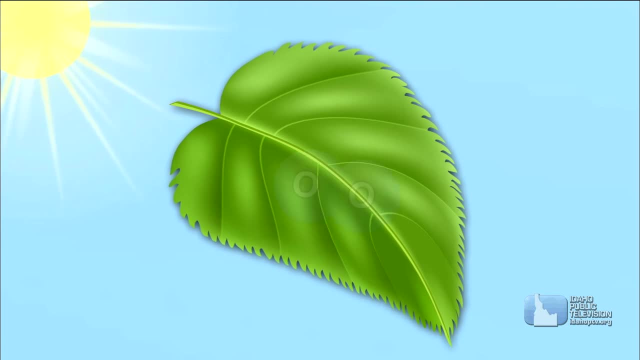 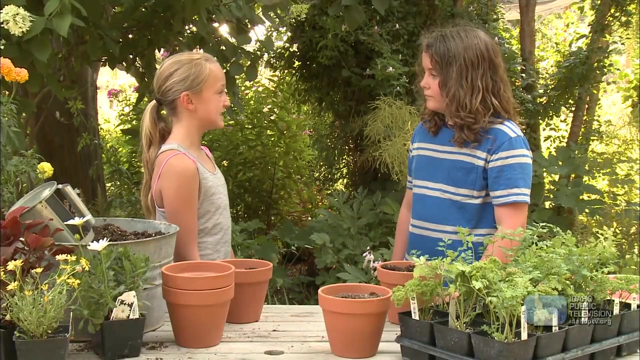 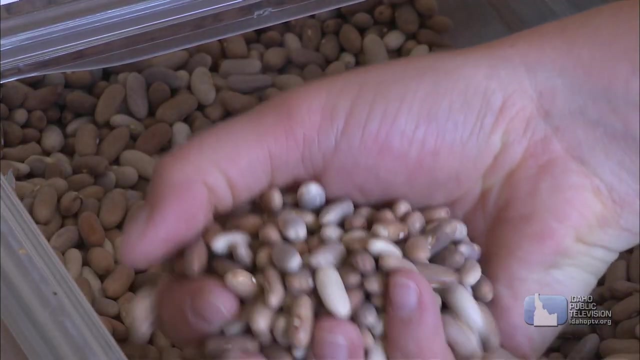 plants release oxygen. That's important because that's the oxygen we humans need to breathe. Wow, that is important. Plants do a lot of things, but one of the big things is providing us with flowers- Flowers. Why are flowers important? Most plants produce seeds. that. 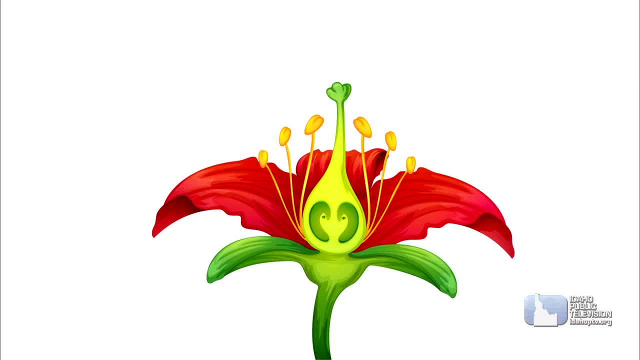 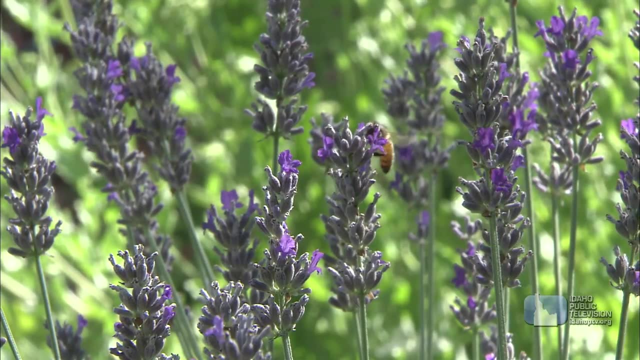 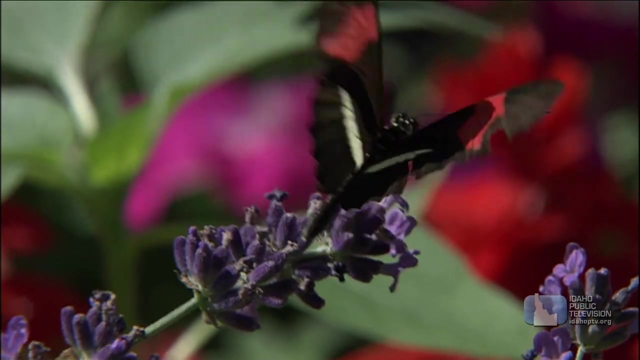 grow into new plants. That's how they reproduce. Inside a flower are the pistil, the stigma and the stamen. The flower also creates pollen, Insects, animals. even the wind can move pollen from one plant's flower to a different plant's flower of the same species. Once this happens, 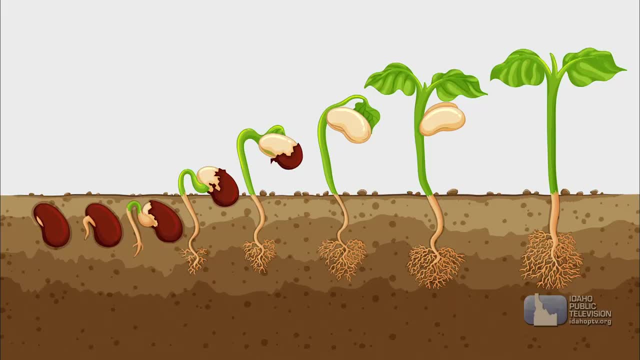 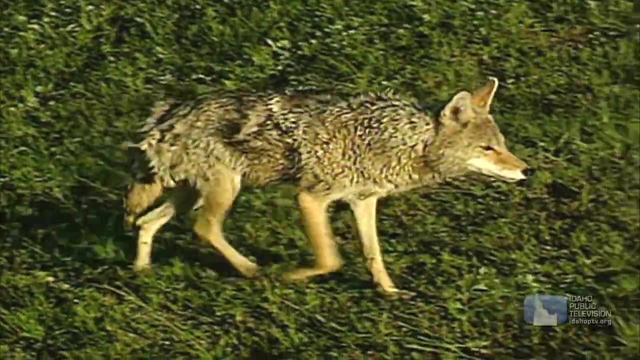 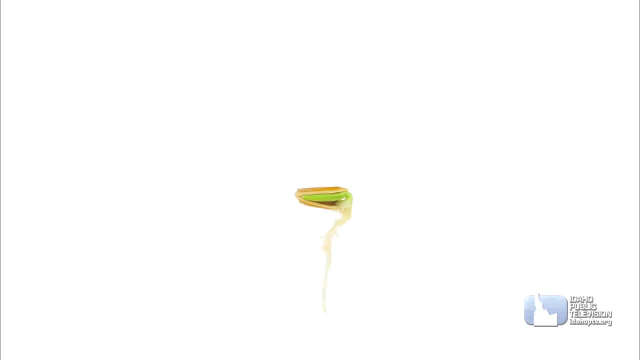 and it's called pollinization. a seed forms. A seed is a baby plant and food wrapped inside a package. Seeds move on the wind or are carried off by animals or insects and fall to the ground. In the ground they germinate or begin to grow. They soak up water, which splits open the outer. 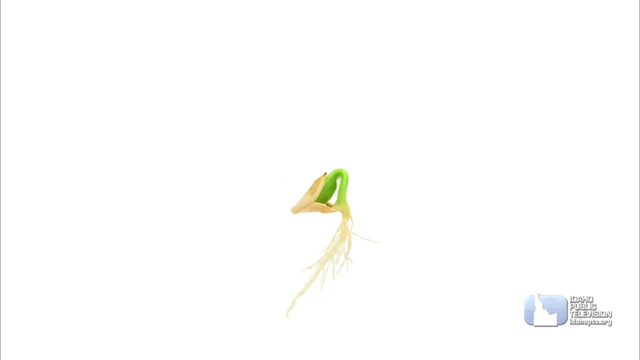 shell Roots push down into the soil and green shoots break through the soil toward the light. Once the shoot turns green, it starts putting out leaves and flowers and the whole process starts all over again. Seeds are important because in some plants the seed comes from inside the fruit. 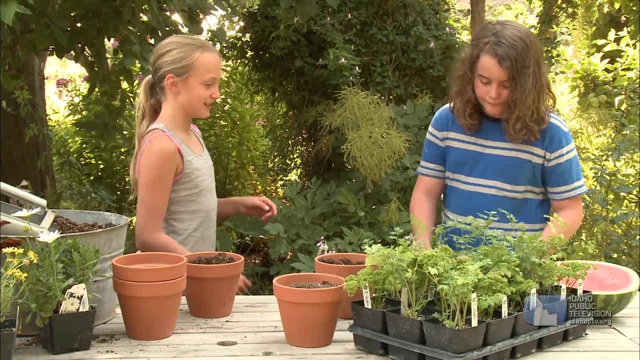 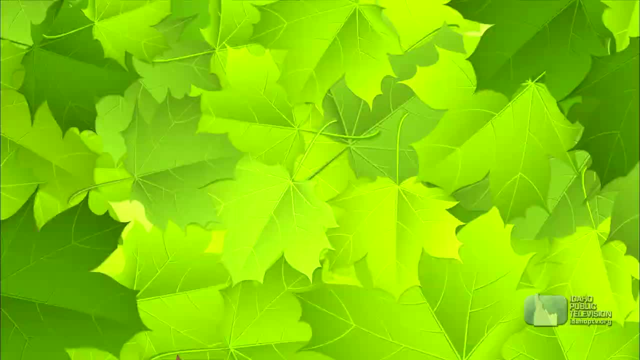 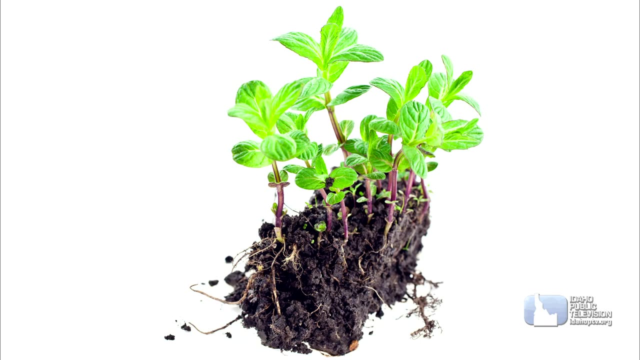 and vegetable we eat every day. Really, Hand me that watermelon. You can see the seeds inside. Wow, that's really cool. Not all plants use seeds To grow copies of themselves. mint sends out small shoots which root into the ground.